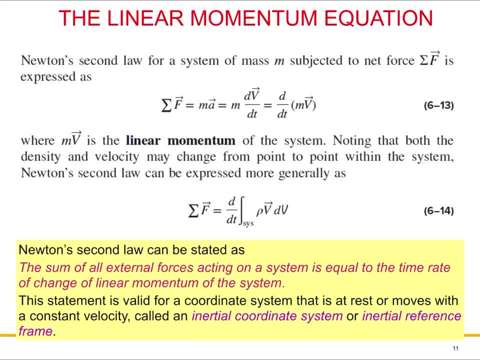 So what it is? We'll try to derive this momentum equations because we're going to use it for almost all of the problems. So initially we'll have a discussions regarding the Newton's second law of motions. We all know the Newton's second law of motion. This is a equal m a and we discussed this earlier. So a is the accelerations and m is the mass. So acceleration you know it is at the rate of change of the velocity. So this is here the rate of change of the velocity. So what we can say we can put m here and this is the derivative term d dt over m p. So m p you all know this m p this is actually the momentum the mass and the velocity the multiplication of the mass of the and the velocity. This is actually the linear momentum of the system. So what we can say this. 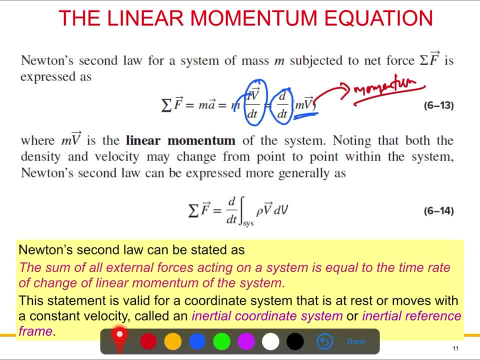 This Newton's second law you know it's telling about you know the rate of change of the momentum. 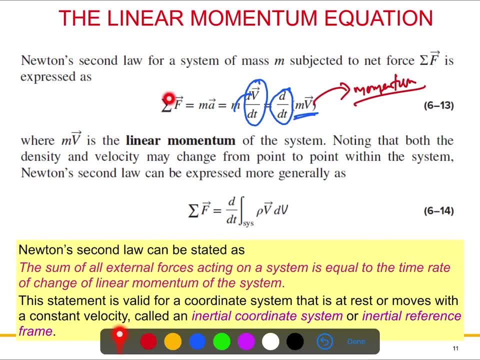 It is equal to the sum of the forces acting on this. So in other words we can we can say this is you know the Newton's second law of motions. We can state it like this is actually the linear momentum formula. Actually we discussed it earlier. So what we can say here is the rate of change of the linear momentum is sum of or is equal to the sum of all the external forces acting on this of the system. Anyway so 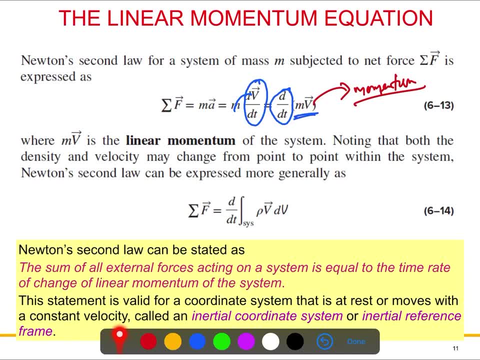 this is the expressions we already know. Now if we know that the the density and the velocity maybe this is variable it may change from point to point within the system. So we have a system so the density and the velocity it could change from point to point. So then Newton's second law of motion can be expressed. So we can say that the density and the velocity of the velocity of the system. So we can say that the density and the velocity of the velocity of the system. So we can state it like this. It is d over dt and the rho V dv. We just use the formula mass you know mass 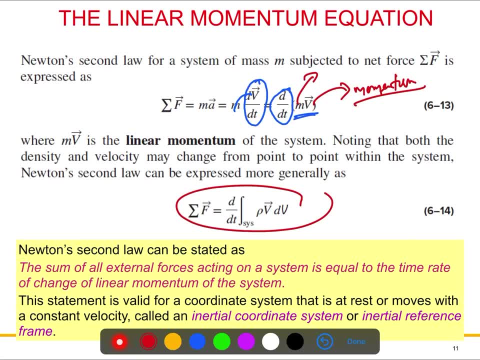 here it is equal you know the density and rho dv. Anyways so now here you can say this is rho V dv. 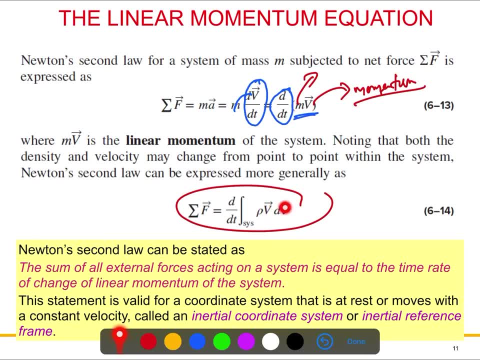 This is the momentum of the differential element dv okay. Or 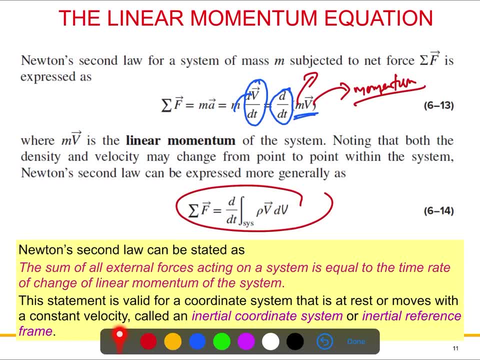 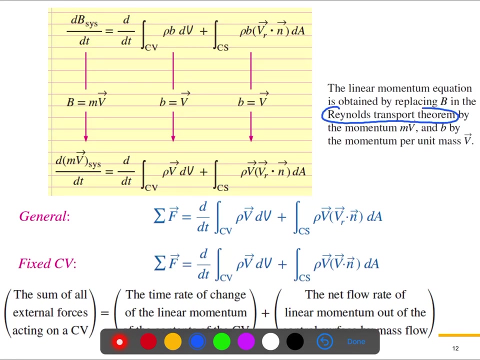 if we say the mass delta m equal rho dv okay mass equal rho dv anyways so now these equations okay this equation it is given mass for a solid or a fluid okay and it is limited using fluid mechanics since we usually use most of the flow system like as a control volume so that we usually do so that means we cannot use it for you know all problems so now to make it easier we'll use a new concept this is called the reynolds transport theorem it is in chapter four in your from your book you will see the reynolds transport theorem especially for moving um system and a fixed control volume it is you know you can just go to that it is a section 4.6 from your book so from the reynolds transport theorem we know this formula this is uh for the system and we'll convert it into the control volume here this b this is a extensive properties we you know the definition of the extensive property it is um you can say the mass b could be mass energy or you know the moment okay so , b is the extensive property this small b this is the intensive property intensive property okay so 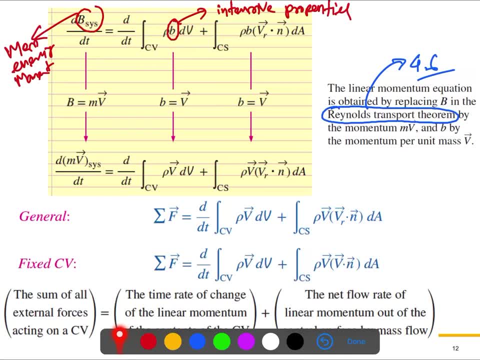 what we will do you can see this is for the control the this um is the rate of change of all the it could be any of these properties okay this is for the control volume this is for the control surfaces 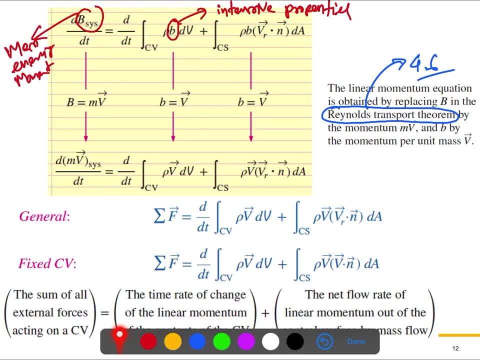 so we will replace this term in this case our intense extensive properties it is actually the moment mv so in the state of b we replace mv the ex intensive properties here we have the velocity is the intensive property here if you if you are wondering what is the definition of the intensive extensive properties go through the lecture one or two and you will get the little explanation of the explanation there so we substitute the value b equal v b equal b in the this two part of the right hand side then you see we'll get it as d dt mv for the system equal d dt rho v dv and this and you can 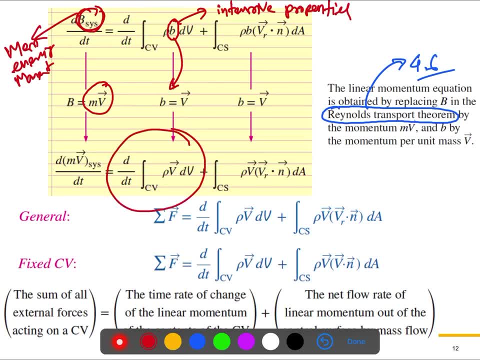 remember it was the final first term we already obtained uh if you go through the first video then you say this is uh the the body force acting on this um on the control volume throughout the control volume and this is now the surface forces we got it from the renal transport theorem so that means we can say here look the left hand side okay the left hand side of this equation this is equal 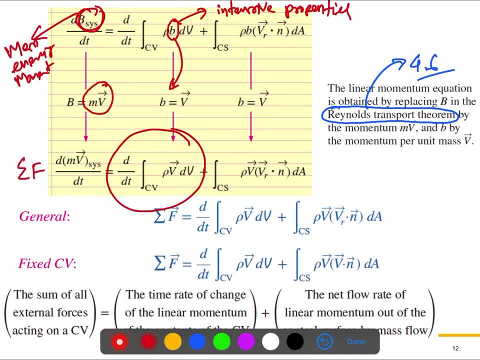 to sum of the wall forces acting on this control volume so the general form then we can write okay if this is equal to sum of the wall forces acting on this system so this is equal now d dt you see 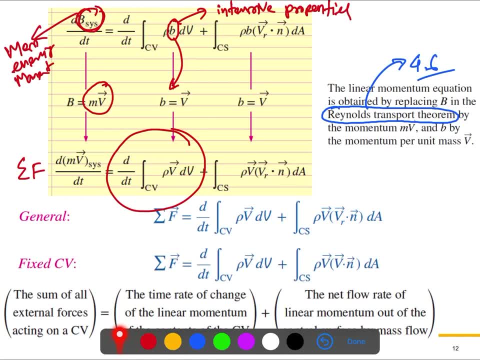 this control volume rho dv for control surface vr dn so this vr this is the relative velocity okay we can calculate this this vr this is actually the average velocity minus the velocity of the control system okay this is the relative velocity to the control surface okay and v is the fluid velocity b this is the fluid this is the fluid velocity so now we can uh for the fixed when it is the general one that is the relative velocity but if we consider a fixed control volume so then we do not need any more relative velocity then it will be just v and you if you look here at this sections so we have rho v vr and d a if we write it down like this rho you know v r into n d a this is we can say this is the mass flow rate through the differential area d a anyways so we have got this is the final term for a fixed control volume this is sum of a p called this and this so this is sum of all forces this is the rate of change of the linear momentum which is um it is due to the body force and this is the net flow rate you know the net flow rate of the linear momentum out of the control surface by mass flow so this is uh for the you know control surface this is for control volume so we have got the for the fixed control volume this is the final term um we actually use for any problem 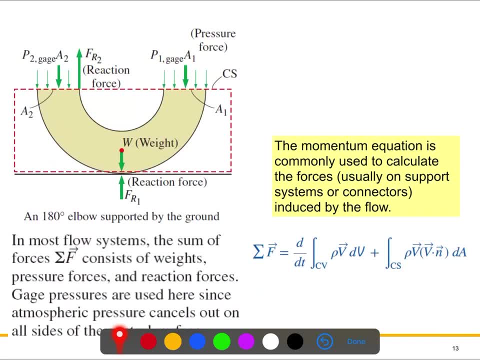 so now here this is some explanation um like uh we have a 80 degree angle elbow um grounded we have some reaction forces here so the momentum equation we're using uh actually um you can see for this support so weight gravity due to the gravity you know weight is acting downward direction this is the reaction force so this is reaction force fr1 and fr2 you know the gas pressure here gas pressure here this is the dotted line is the control surface this inside it is control volume so here it consists the f it consists couple of things the pressure force you see the pressure acting here into the area this is the pressure force this is the pressure force what else we have we have the reaction forces okay so also the weight so there's the sum of all forces acting here um so when we'll solve this problem uh actually uh you know we will solve some problem 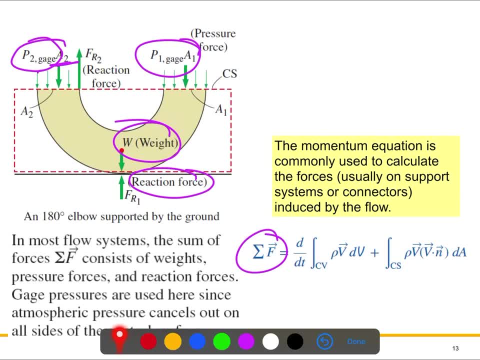 like this and then we'll explain actually how to use this in um and how to apply these equations so now some special cases uh what do you 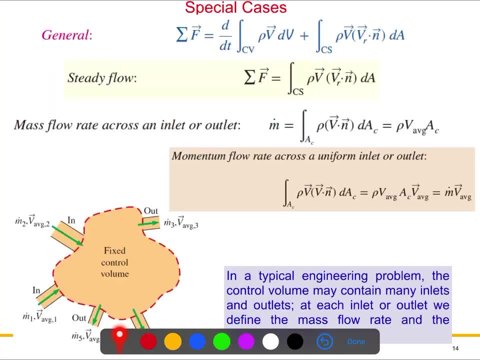 we showed here this is you know uh for the fixed control volume so now for special cases let's say for a steady flow we'll talk about the steady flow so steady flow means if it is the control volume so the mass um inside the control volume or the the moment inside the control volume it will be constant it will not change it has number of inlets number 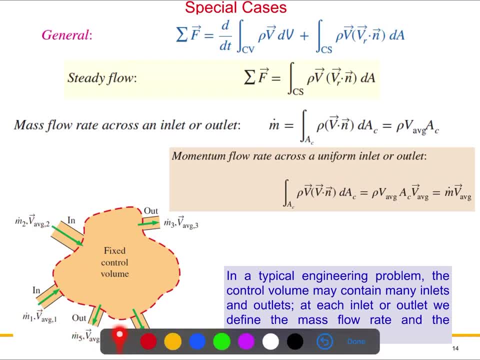 of outlets you can see so it's coming in uh going out but as it is the fixed control volume for a steady case the what we can say the the mass of the moment inside the control volume it will be fixed so that means it will not change with respect to time but this is actually the rate of change with respect to time in the control volume so what we can say here when it is steady case then it will be zero for a special case the control volume remains constant okay the amount of moment in the control volume remain constant so